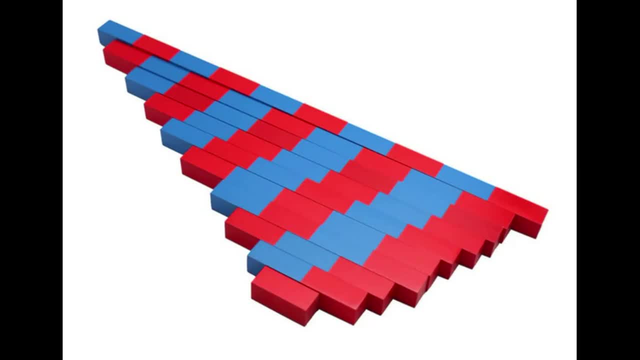 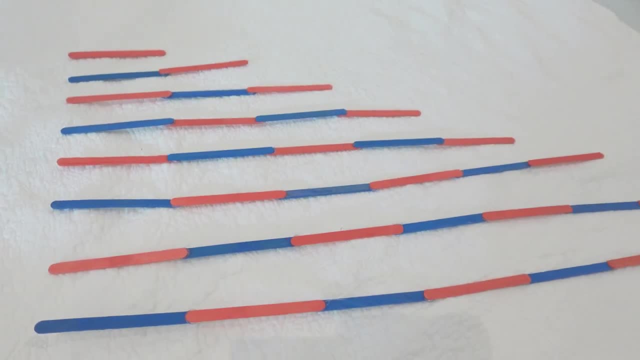 of blue and red sticks. I'm going to be using these two. I'm going to be using these two blue and red colored wooden rods that are arranged in a stair-like pattern, which visually shows the child the concept of getting bigger and help the child practice counting in a concrete way. 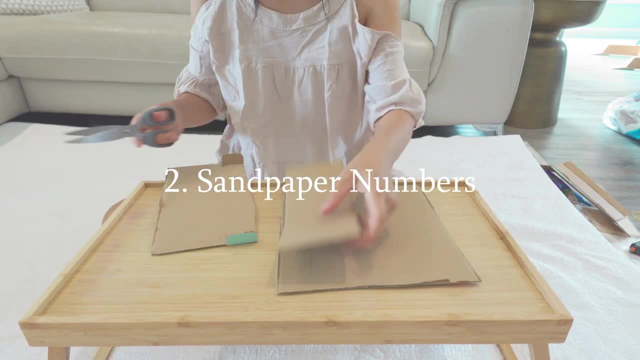 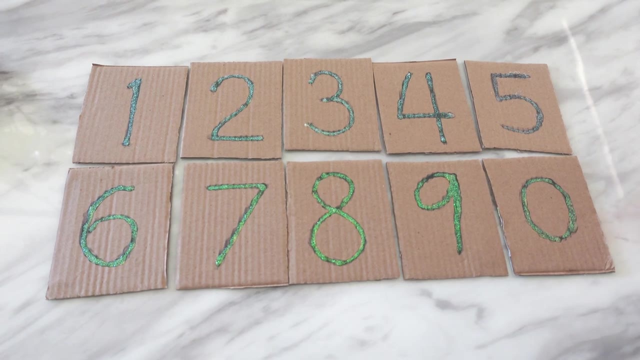 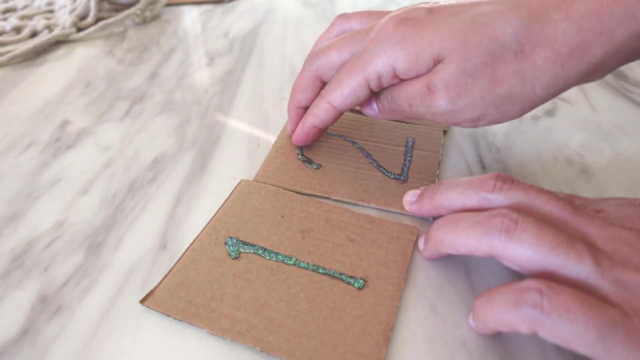 The second activity I'm going to make is Montessori sandpaper numbers. It's designed to teach children the symbols that represent each number, allowing them to visually identify any numbers from zero to nine. Children use their tactile sense of touch in order to feel the rough sandpaper on each board tracing out the numbers. This helps children make the. 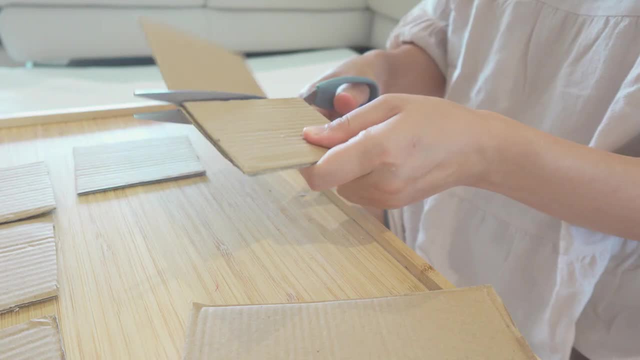 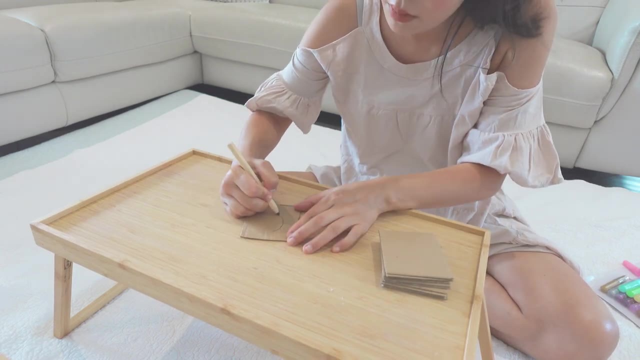 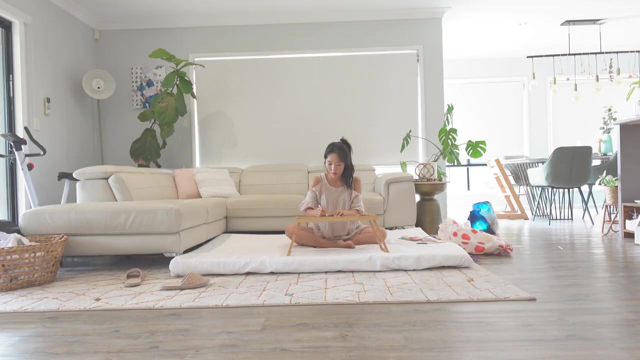 connection between the concept of numbers and the symbol, and it also prepares them for writing. The Montessori sandpaper cards are super easy to DIY at home. All you gotta do is just cut out ten pieces of cardboard, write all of the numbers on the cards and then go over. 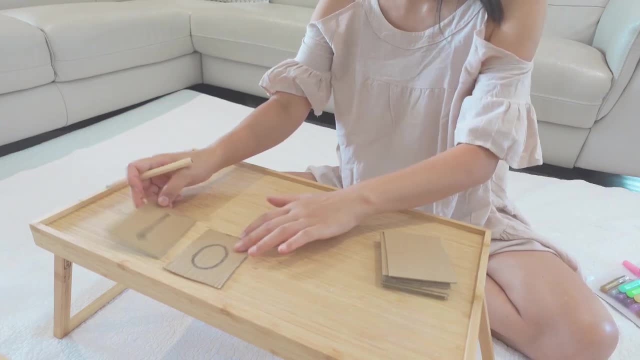 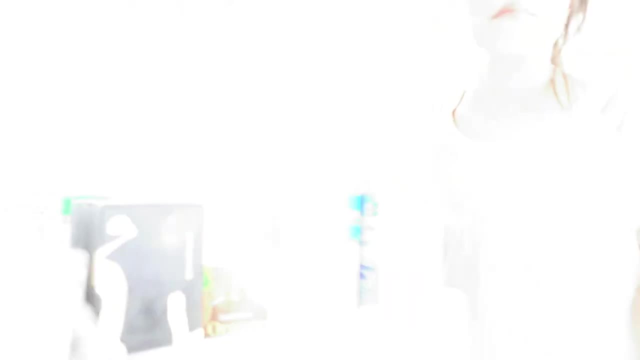 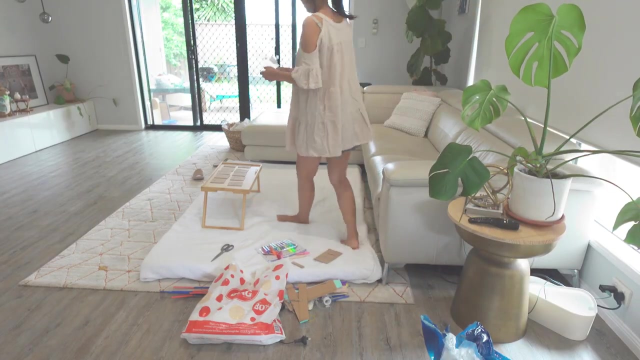 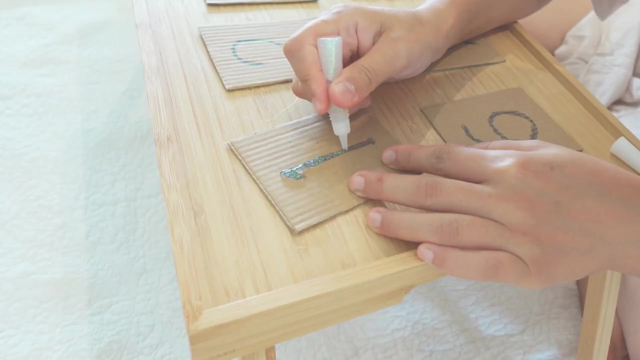 it with some glitter glue and let it dry out. You can also use a very fine grade of sandpaper and cut out numbers, but I just wanted to use what we already have at home. Now I'm going to use generous amounts of glitter glue over it to create that raised. 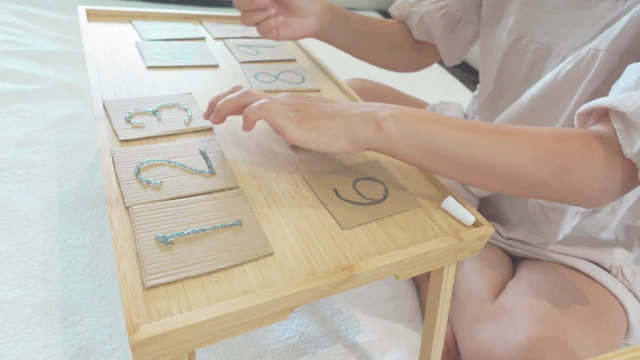 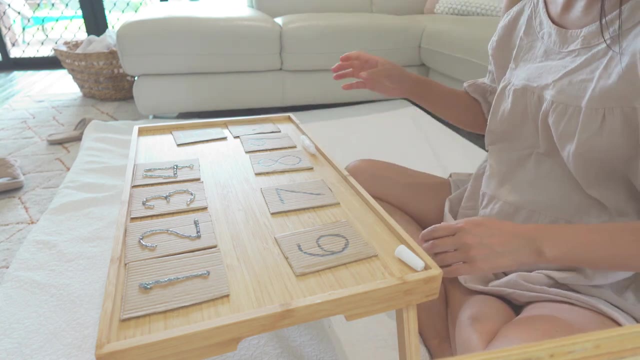 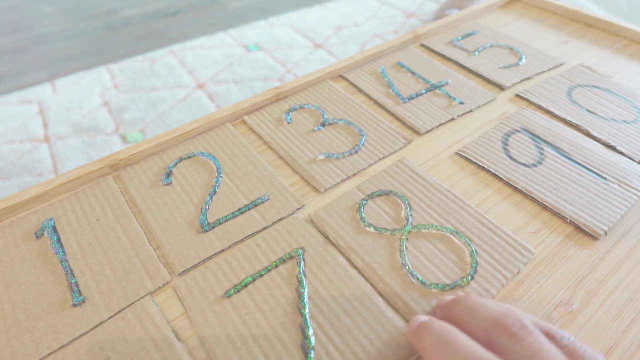 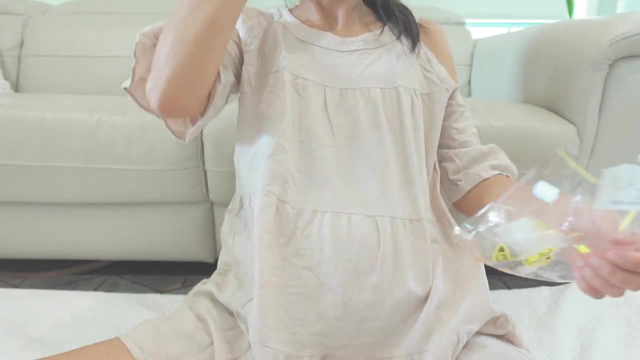 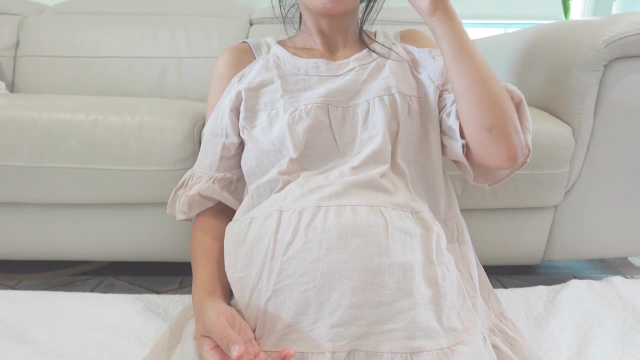 texture like sandpaper, so that Alina can trace each number with her fingers. So, basically, the first thing that I'm going to do is to just like a fingerboard and I'm just going to put the opposite end side in. Now the next activity I'm going to do is to cut out the 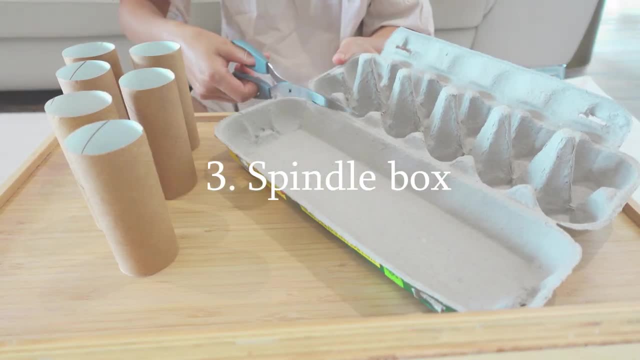 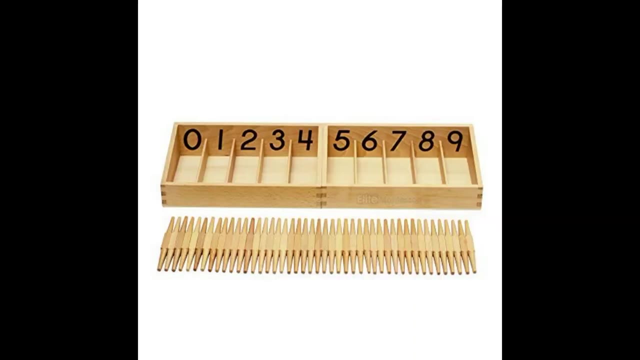 other letter, letter…, is a Montessori spindle box. The spindle box is designed for children to place the correct amount of wooden spindles in compartments labeled 0 to 9.. Again, I'm going to make it just up to 5 because I don't want to overwhelm Alina. I'm using 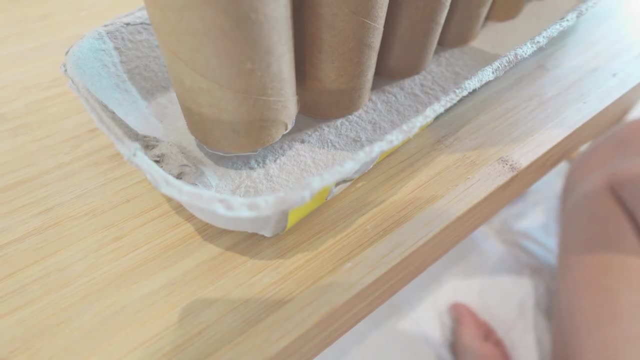 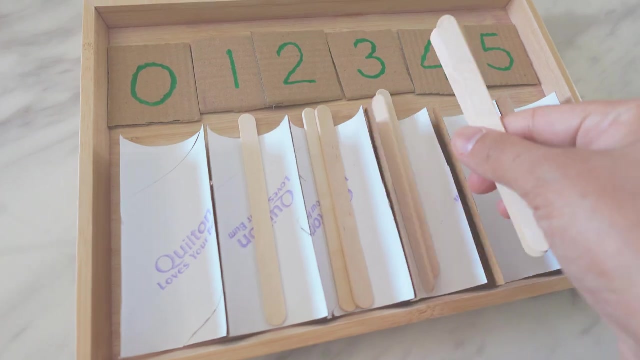 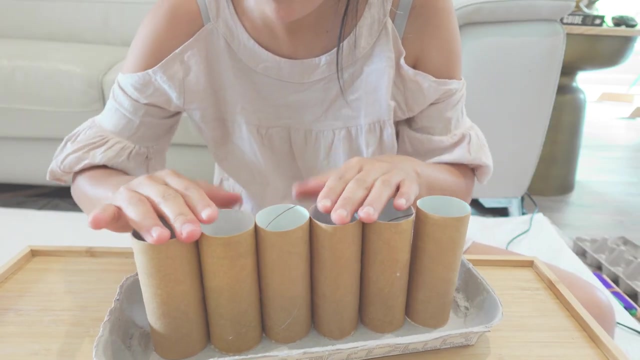 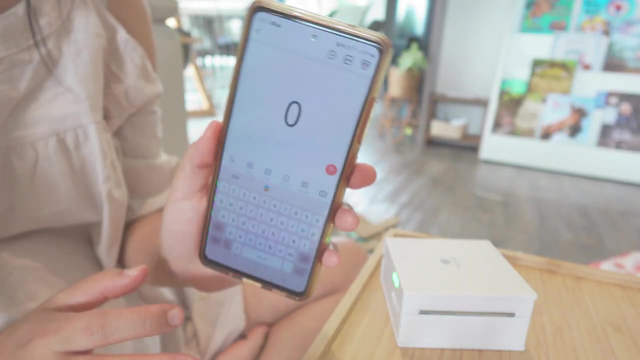 an egg carton and six toilet paper rolls to create six compartments from 0 to 5.. You can cut the toilet paper rolls in half and make it look like this, whichever you prefer. Now I'm going to print out the numbers Again. use what you already. 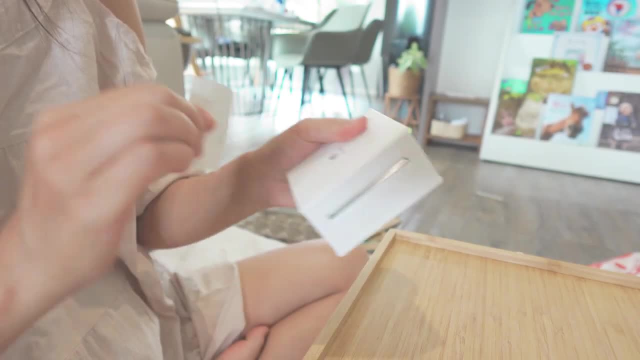 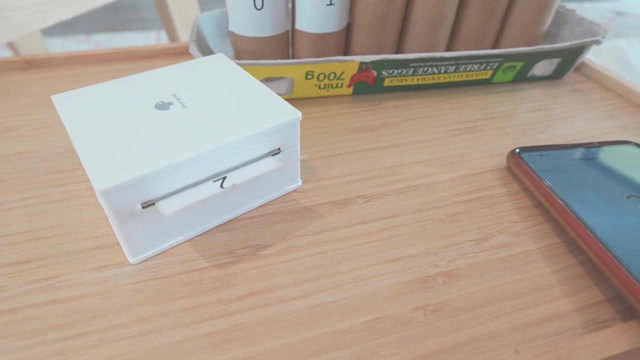 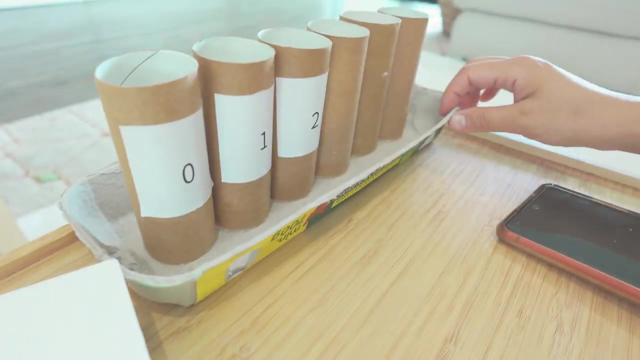 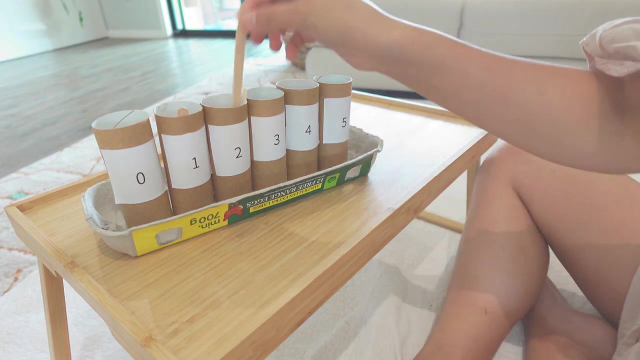 have at home, or you can just simply write numbers in nice big black marker. I just happen to have a label printer at home, so I'm going to use this. The spindle box gives children a muscular impression of the quantities as they collect and bind spindles to place in each section. It's also a great way to 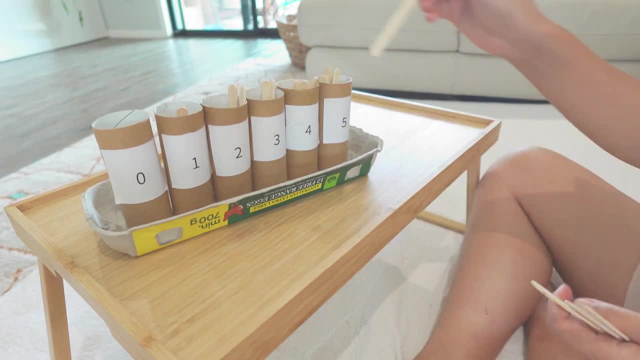 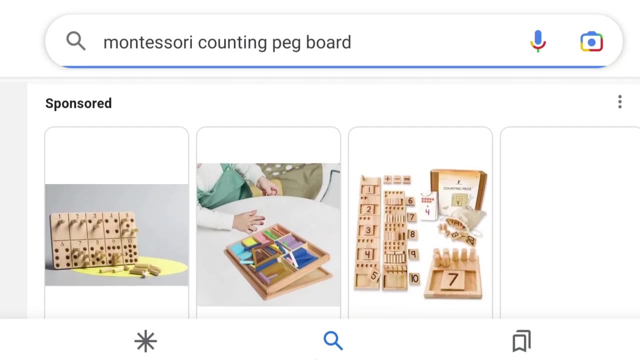 introduce the concept of zero, as one box remains empty while the others are filled. The fourth activity I'm going to DIY is Montessori counting pack board. This material is designed for children to practice once a week. I'm going to use this as a guide for children to practice counting. 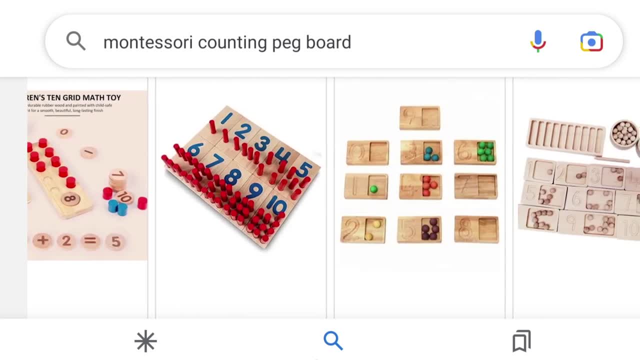 I'm going to use this as a guide for children to practice counting. This material is designed for children to practice one to one correspondence while also seeing the corresponding number symbol. In order to DIY this material, you need some cardboard, box, plastic, bottle caps. 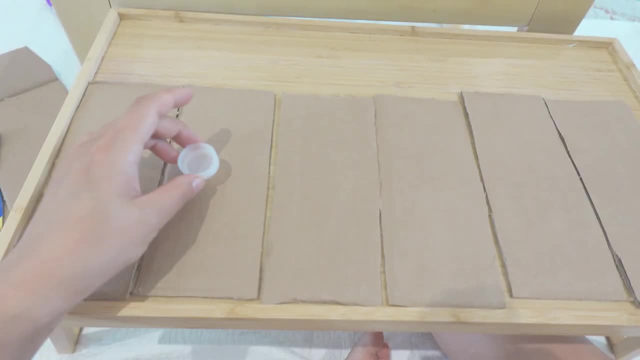 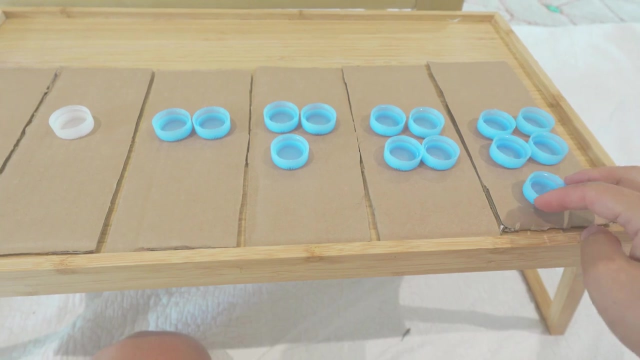 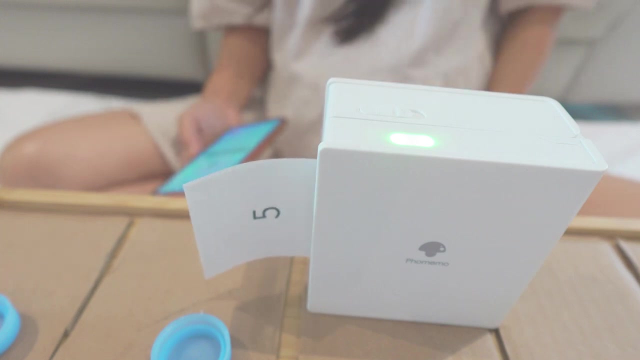 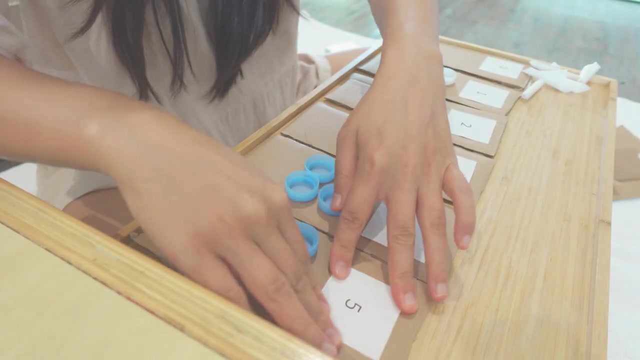 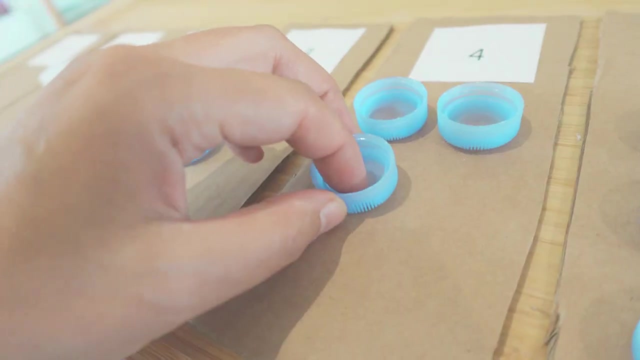 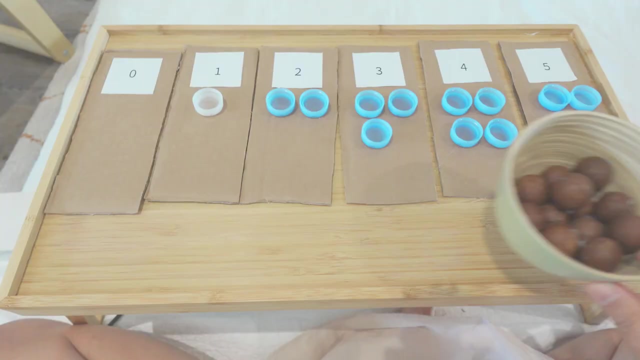 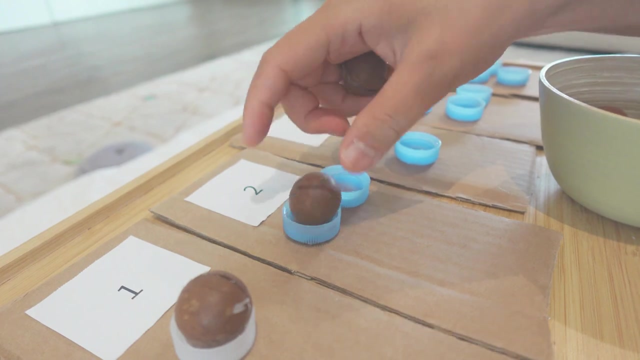 and some counters. I'm making six boards today for numbers 0 through 5, and you also need some plastic bottle caps to create that holes on the pack boards. Now for the counters. we have a ball of macadamia nuts because they just happen to be what we had on hand and they fit. 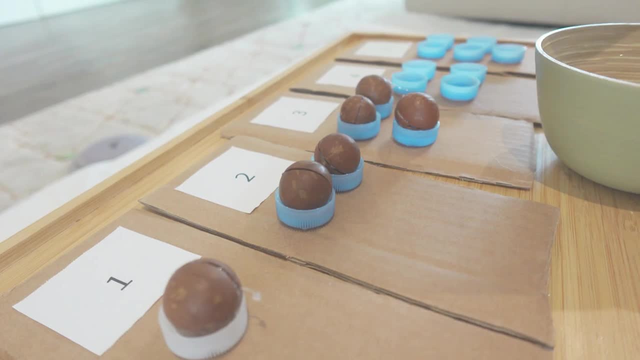 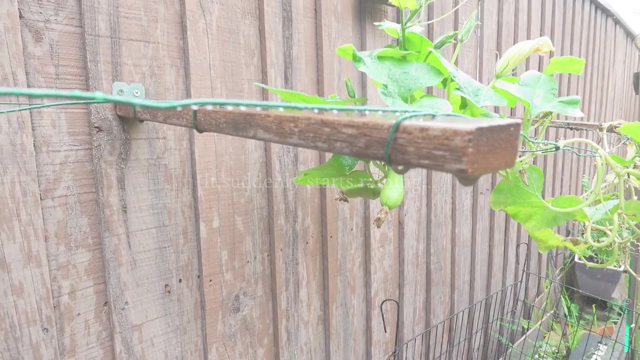 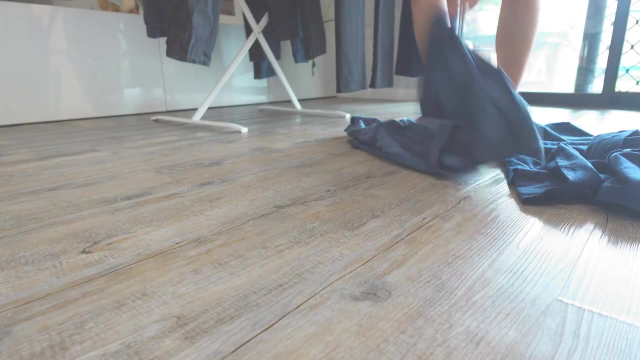 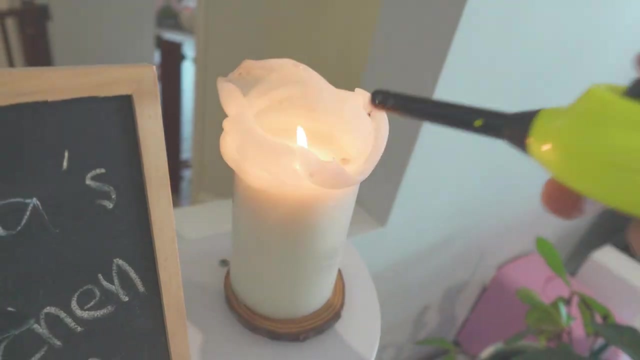 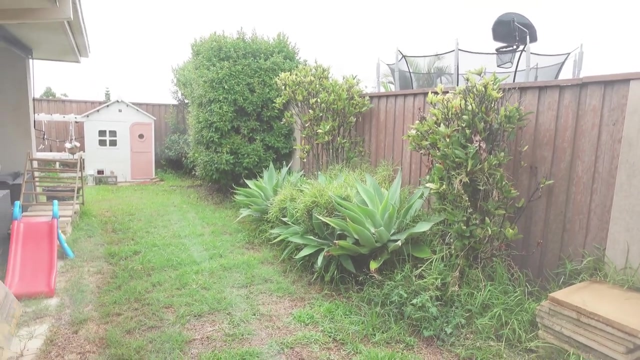 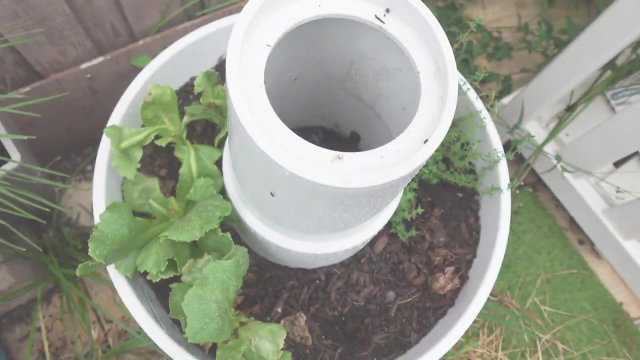 perfectly into the plastic bottle caps. There's just one thing I want to mention before we move on. The purpose of this video is to show you guys that Montessori is for everyone, whether you're on a budget or not. Sometimes we just have to find a way to make it work using things that we already have. 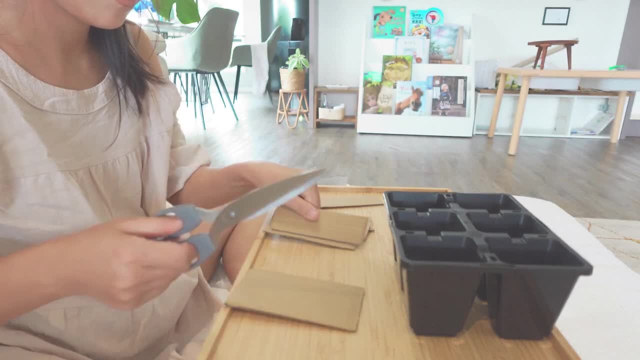 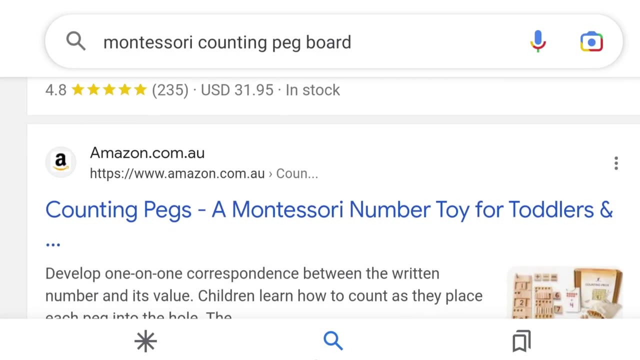 at home. I certainly can't afford all the authentic Montessori materials because, one, they're expensive and, two, I'm not homeschooling Alina, so there's no need for me to purchase those. So I started to DIY a lot of Alina's materials. 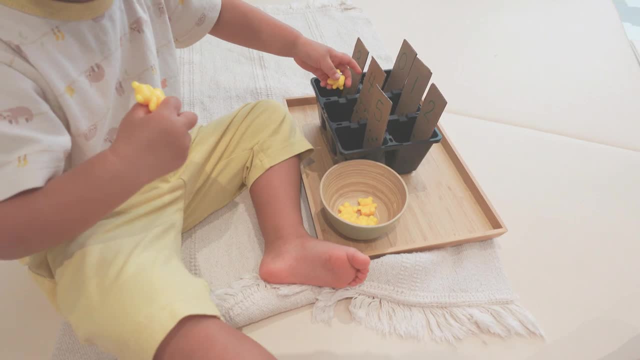 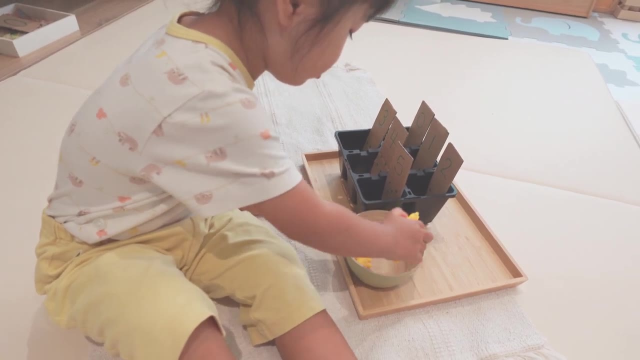 And I found that it's really easy to do and I also found that she loves the material just as much as the expensive version that I just saw online And I'm telling you it doesn't make it any less Montessori because you are making materials. 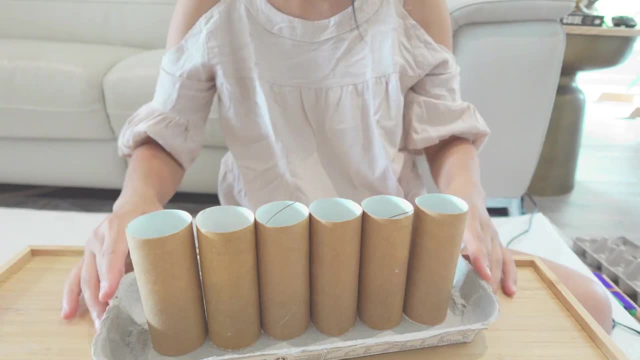 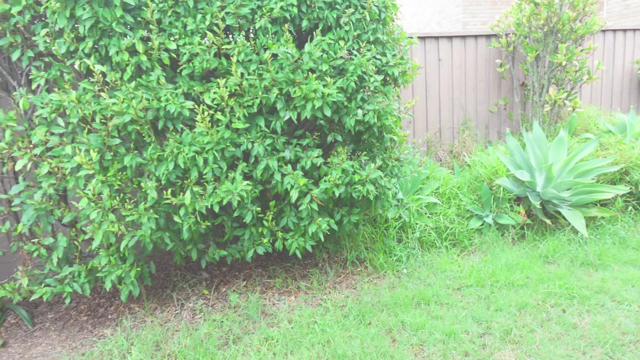 out of egg carton, cardboard box or toilet paper rolls. So I really hope you guys find this video helpful and useful for your Montessori journey And if you like this video, don't forget to give it a thumbs up. Now I'm going to go ahead and show you how I introduced these materials. 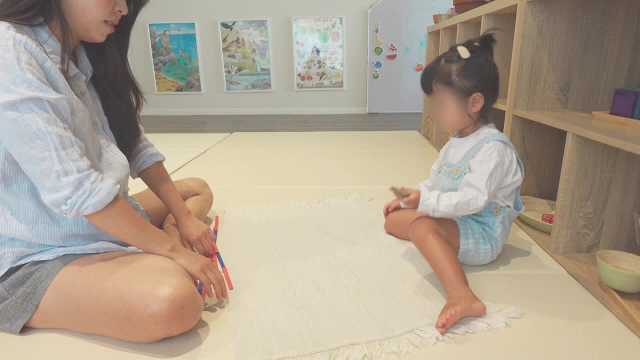 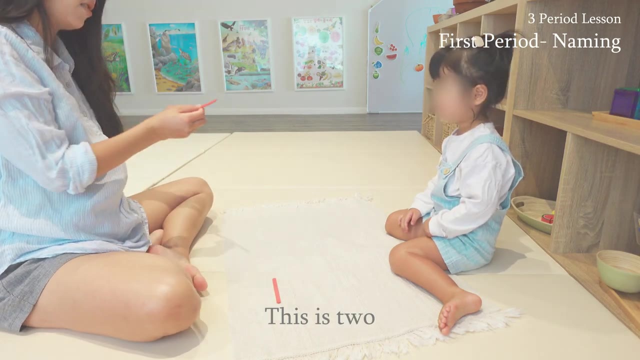 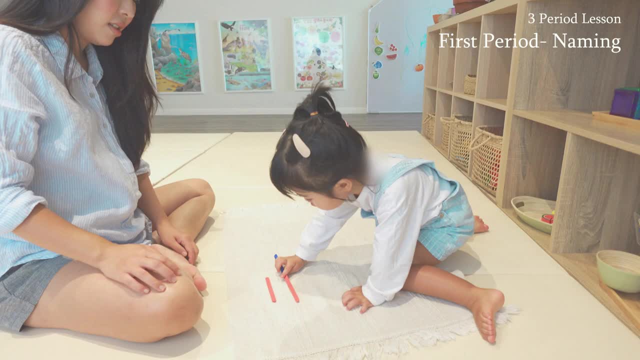 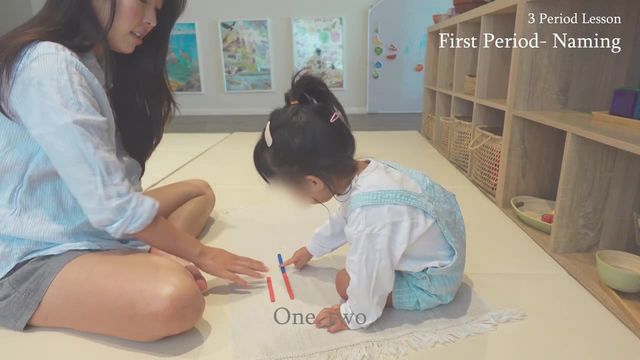 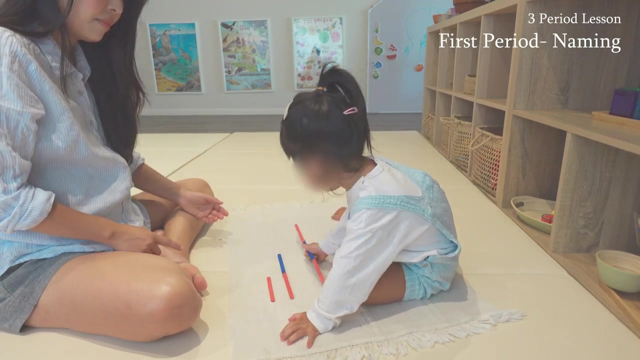 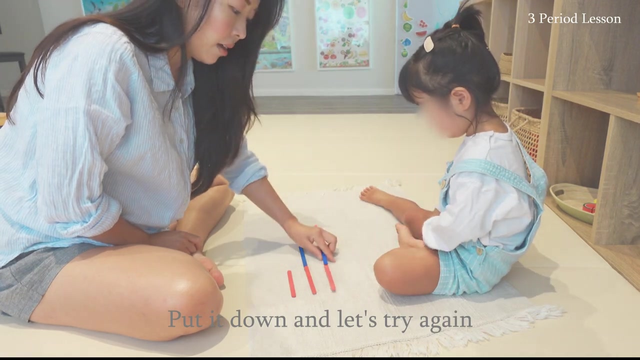 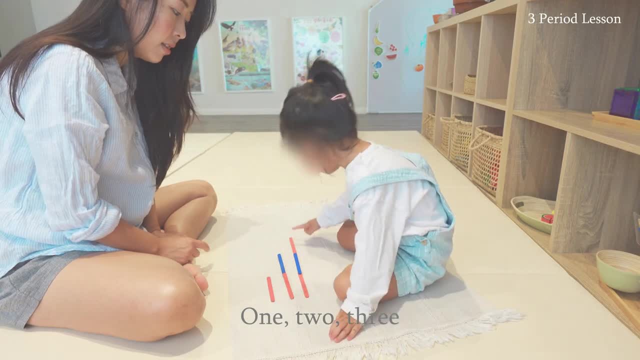 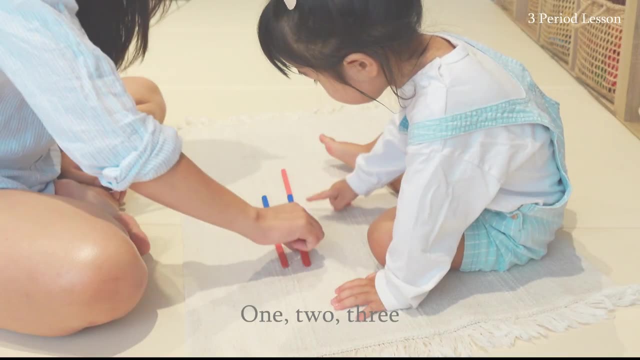 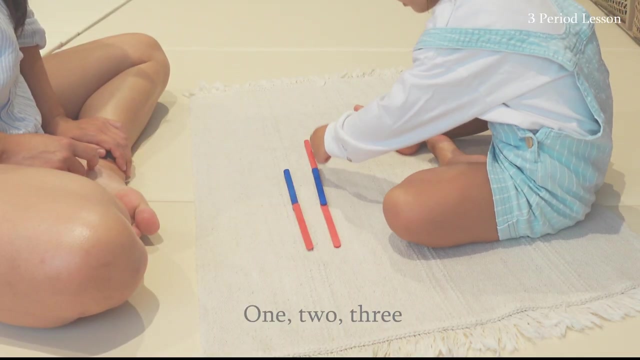 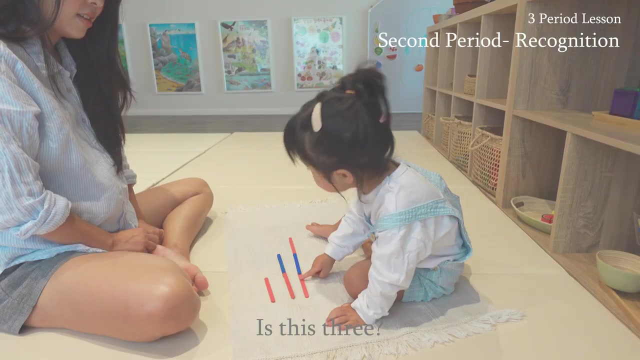 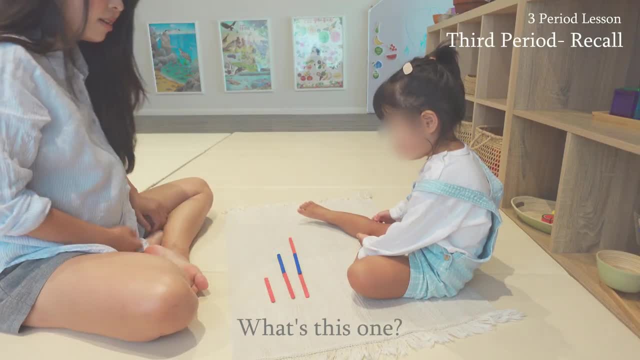 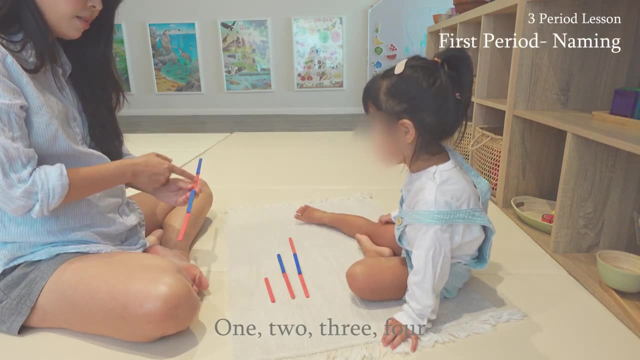 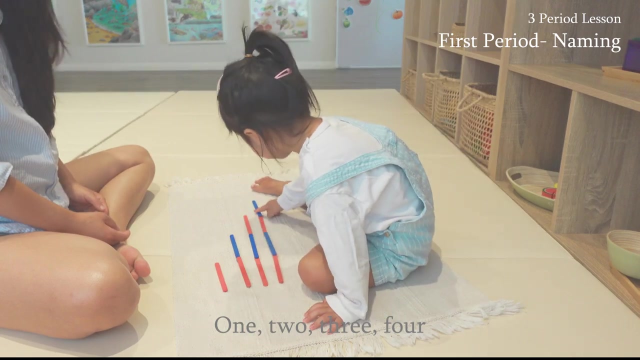 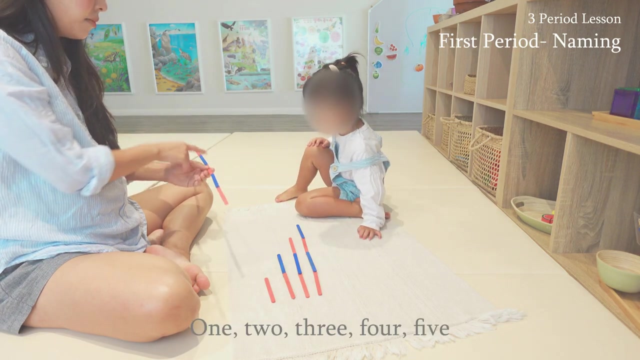 Touch number 3. What is this? 3. This is 1, 2, 3, 4. It's 4: 4. 1, 2, 3, 4. What is this? It's 5: 1, 2, 3, 4, 5. 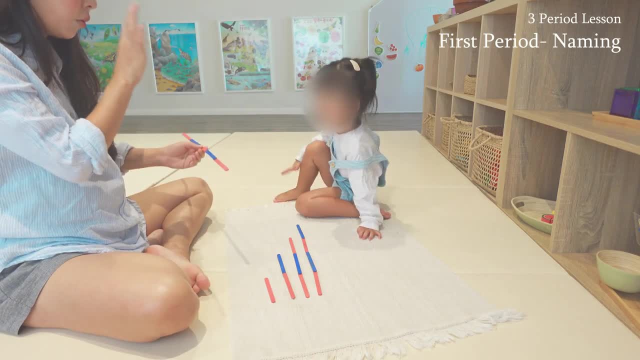 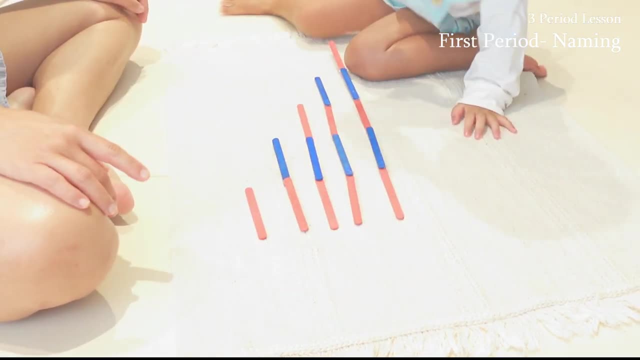 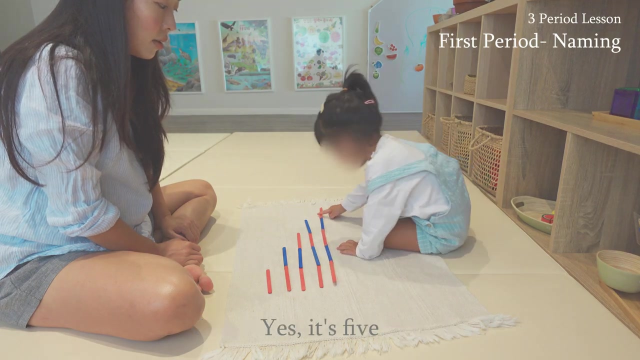 5, 5, 5 is long, right. I'll put 5 here. 5 is the longest Right. 1,, 2,, 3, 4, 5, 5. Arin, do you want to touch number 4?? 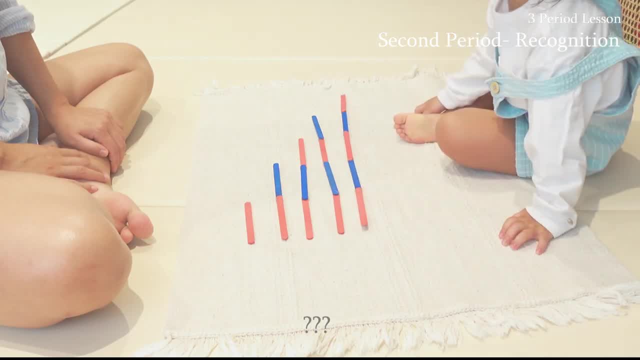 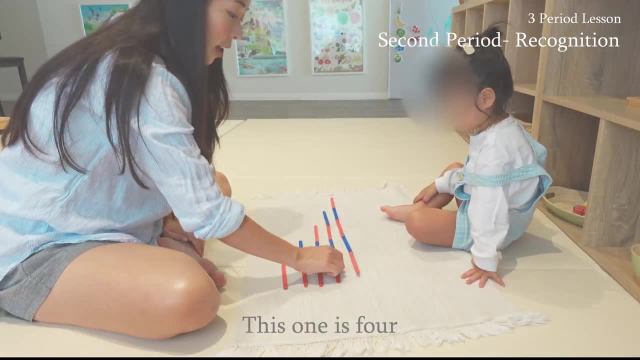 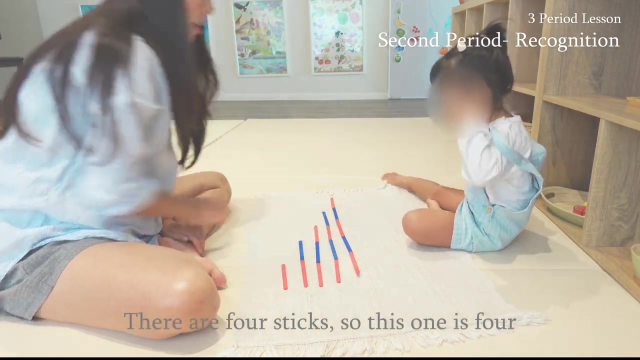 Touch number 4: 5. Arin touched number 5: 1, 2, 3, 4, 5. 4 is 4: 1, 2, 3, 4. 4 1, 2, 3, 4. 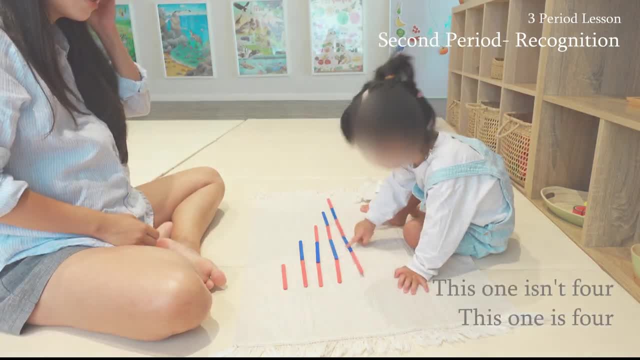 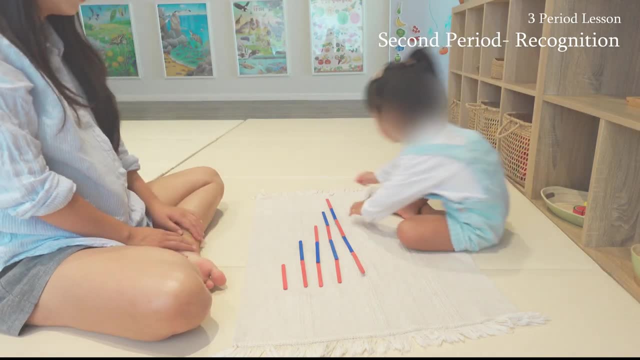 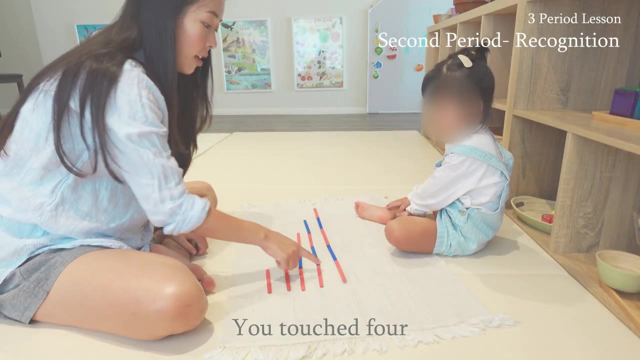 Do you want to touch number 4?? This is 4. That's 5. 1,, 2,, 3, 4, 5. Arin, touch number 3? 3?? Yes, 3. You touched number 4: 1, 2, 3, 4. 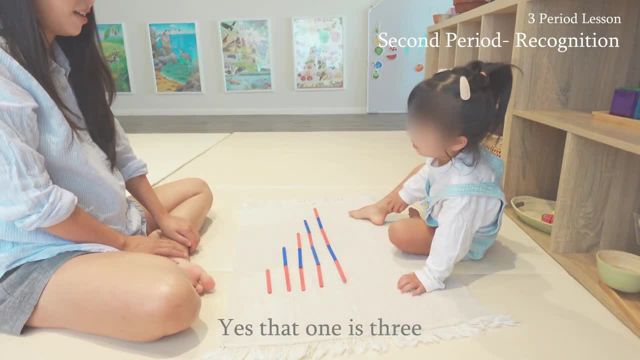 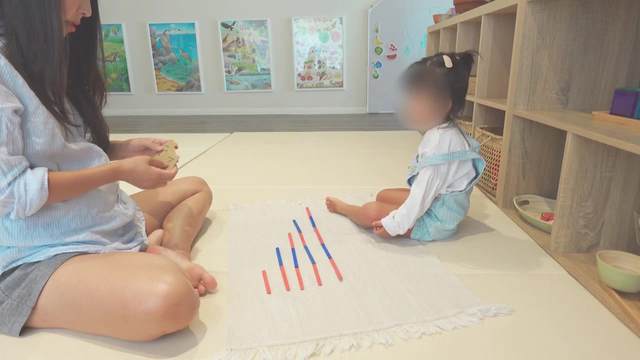 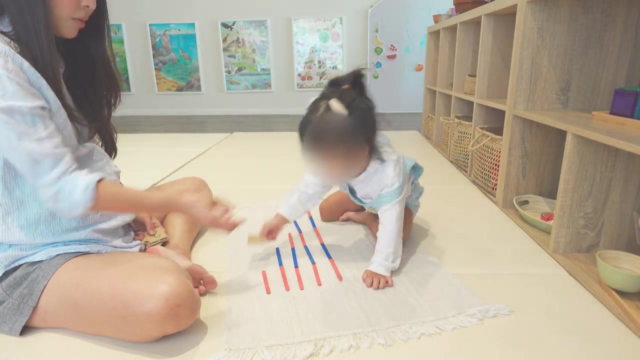 4. Yes, that's number 3. Shall we touch number 5? 5. Yes, Right Now. What is this? 1- 1? Where should I put this Here? Yes, put it next to number 1. 1 Now. What is this? 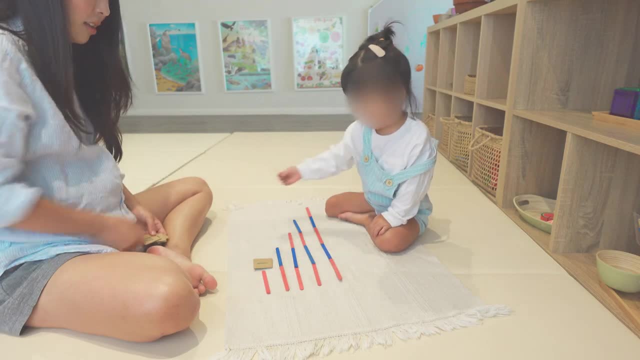 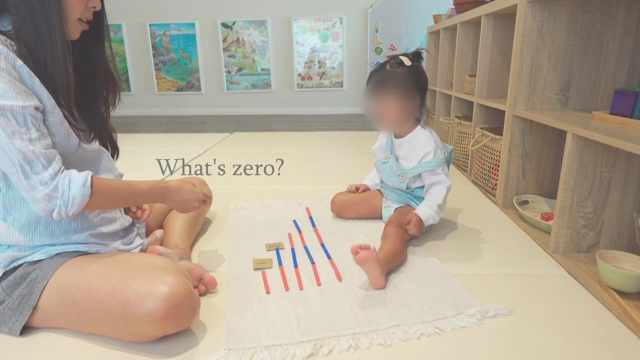 What is this 2? Where should I put number 2? Here? Yes, What is this 0? Yes. What is number 0? Here? Yes, because there is no number 0, You can put it here. There is no number 0 here. 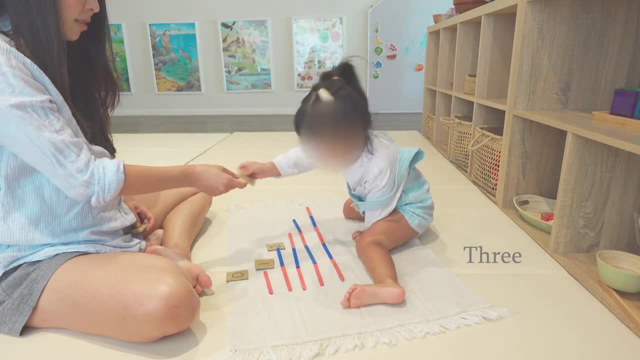 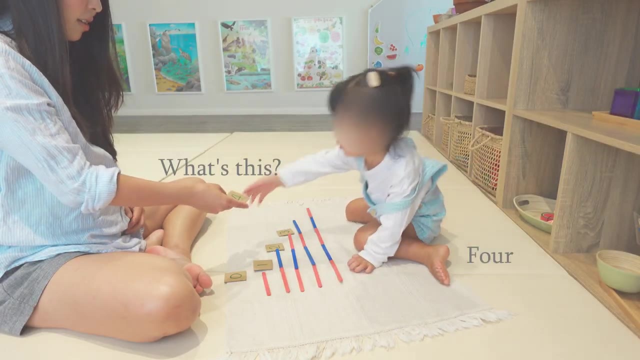 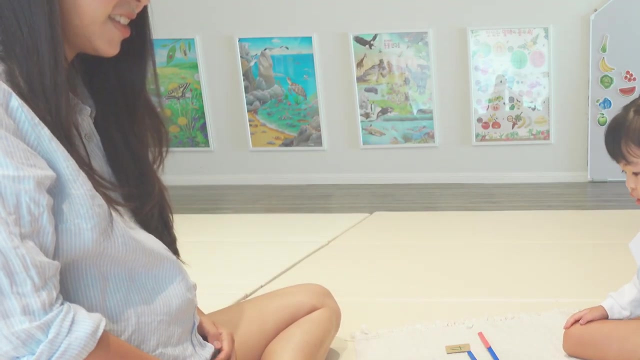 There is no number 0. What is this? 3? What is 3 here? Did you put 3 next to it? Yes, What is this? 4? Oh, 1, 2, 3, 4. Right, So it's 4 because it's 4. 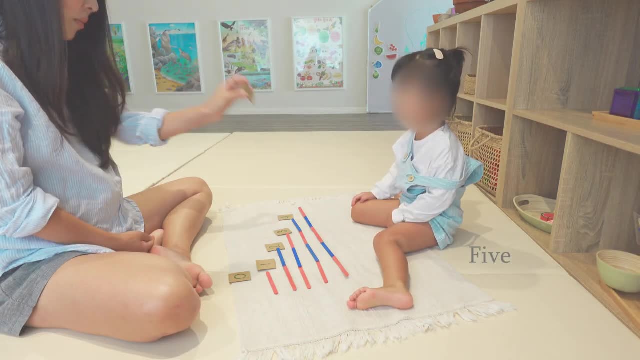 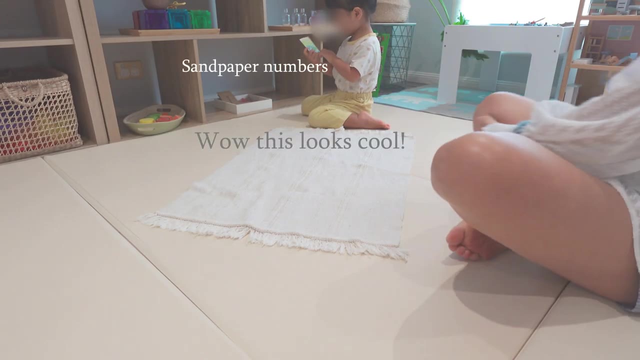 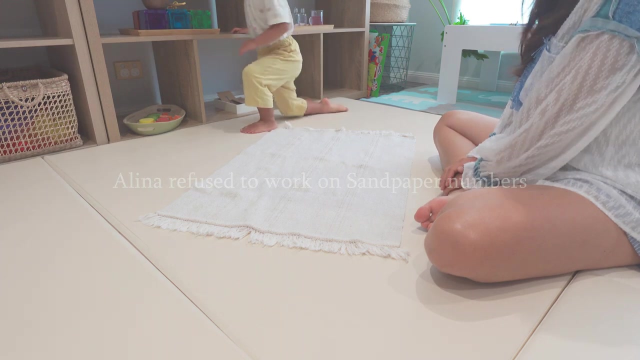 4. Yes, What is this? 0 Yes, Bring the whole tray. Oh, it's so big. I'll show you how to do it. Mom, I don't want to do this Really, I want to do this. Okay, then bring that. Mom, look at this. 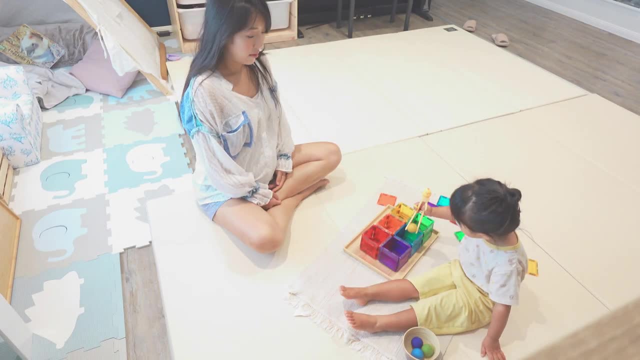 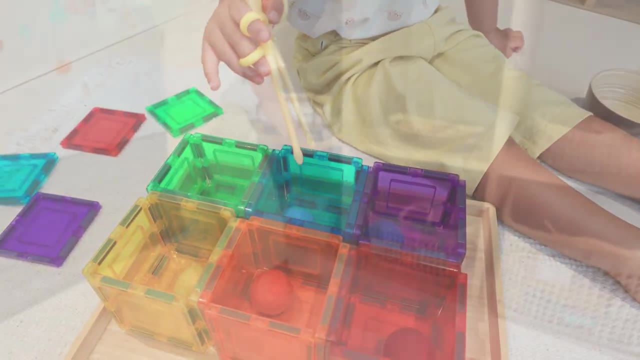 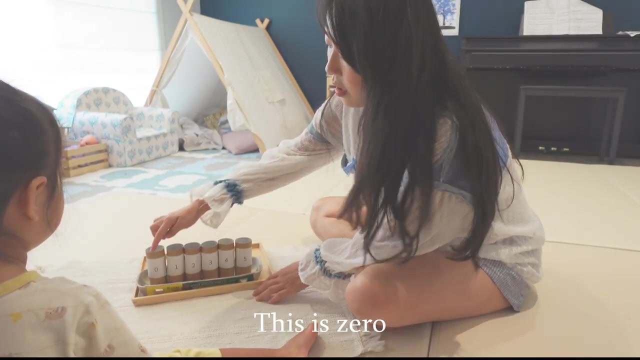 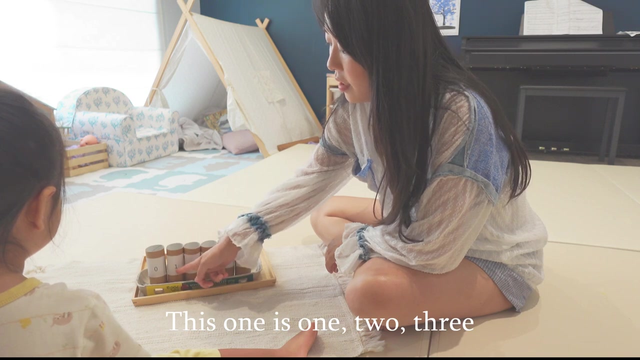 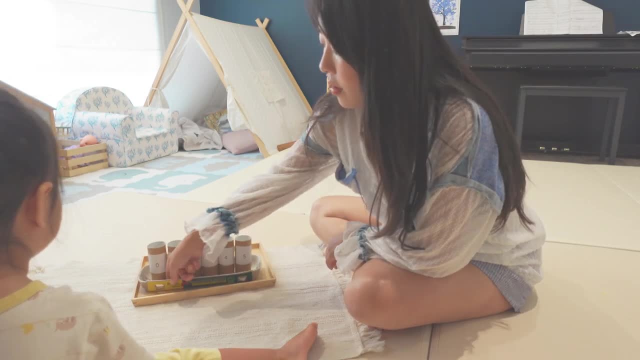 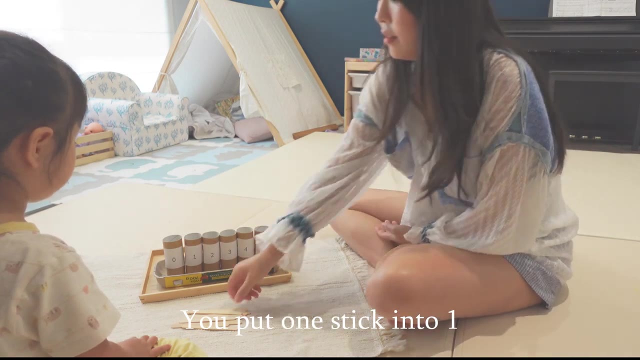 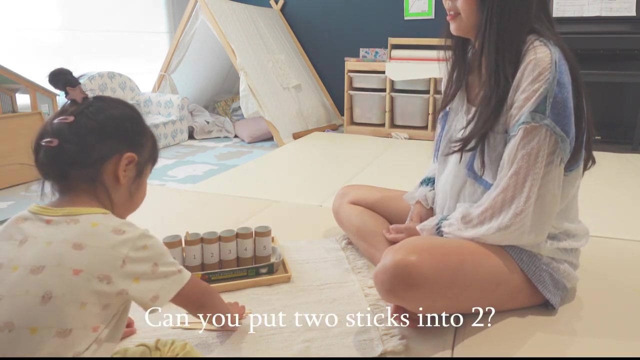 1, 2, 3, 4, 5. There's no zero, There's nothing. You put one in the first one, So how many do you put in the second one? Two, That's right, Arie, put two in there. 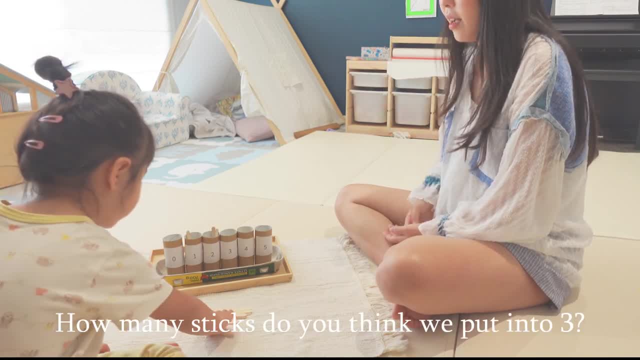 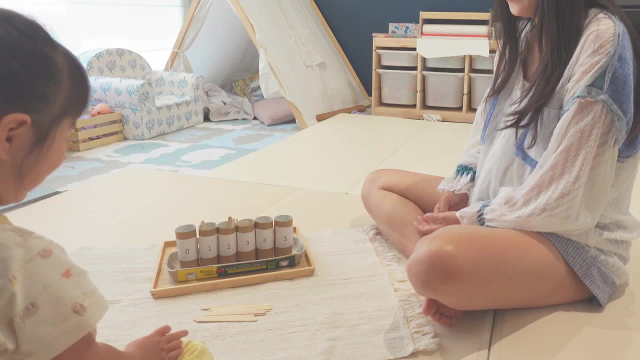 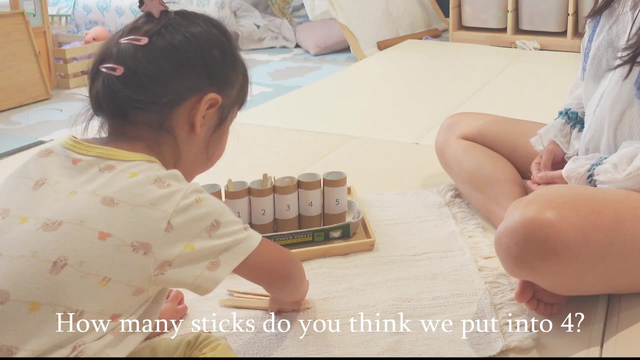 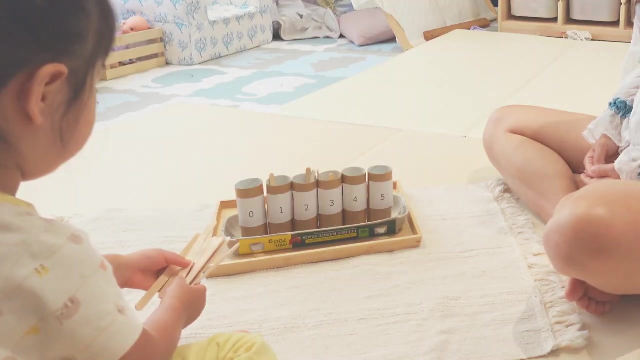 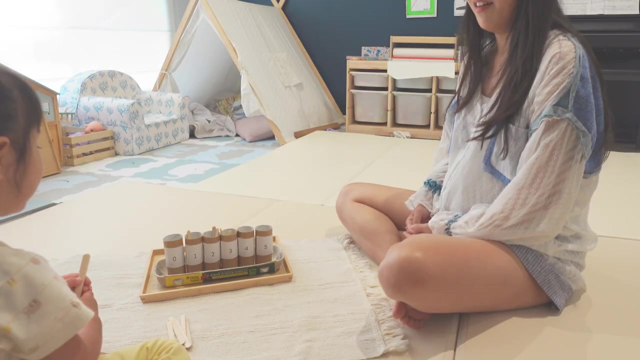 What's this? Three? How many do you put in three? Three, like this, Two, three, That's right. What's this? This is four. How many do you put in four? I don't know. Count four. One, two, three, four. 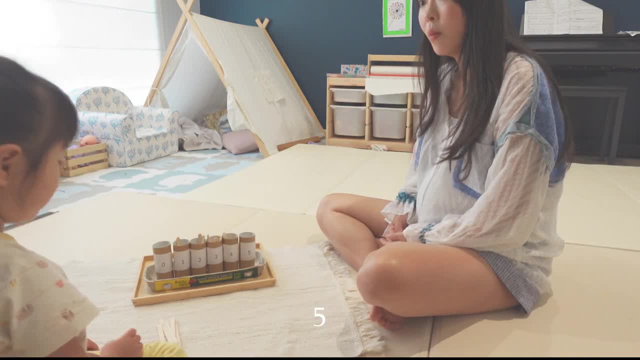 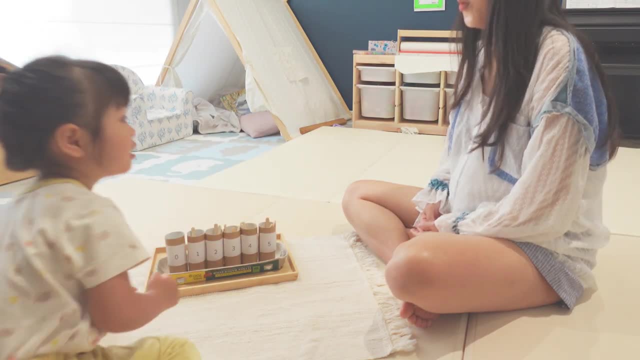 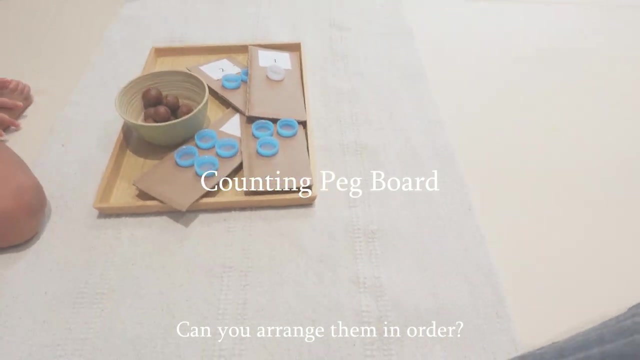 What's this? The number Five, Five. And this is: You have to put five in there. Five, That's right. That's how you do it. Now, Arie, can you put this in your hand? Yeah? 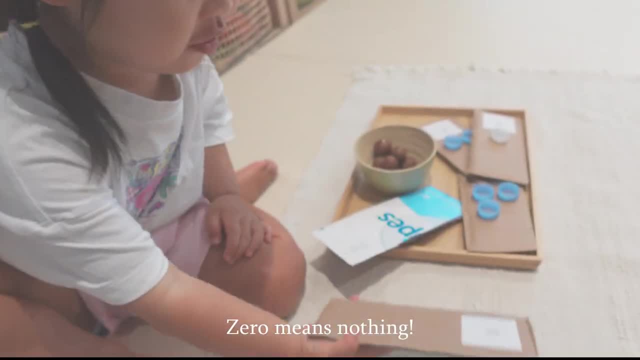 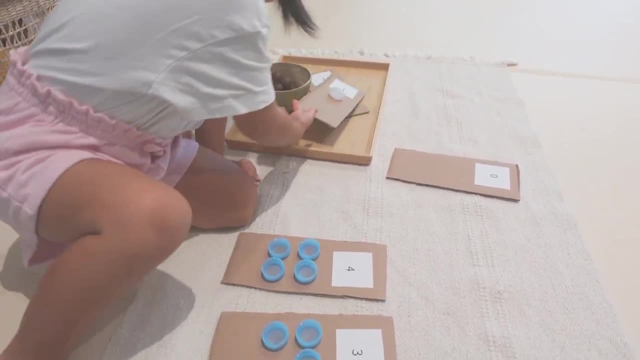 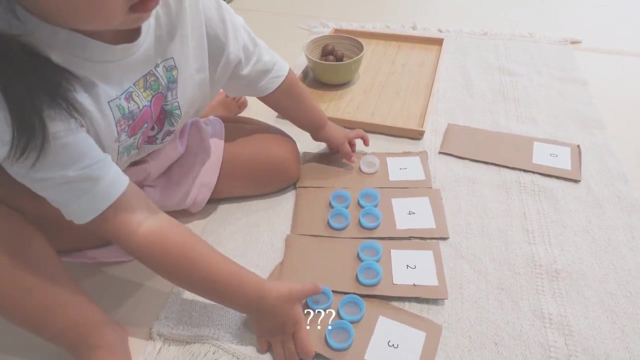 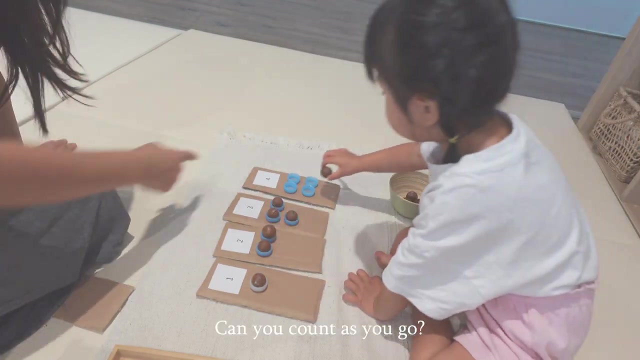 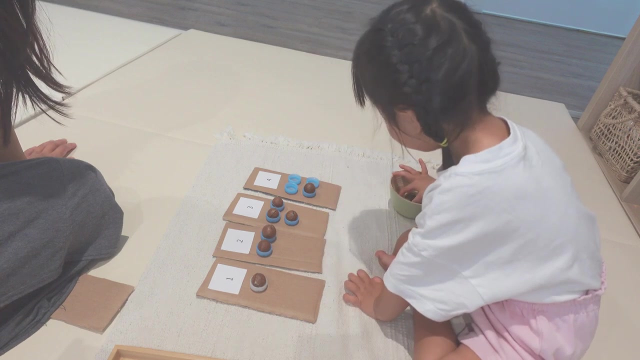 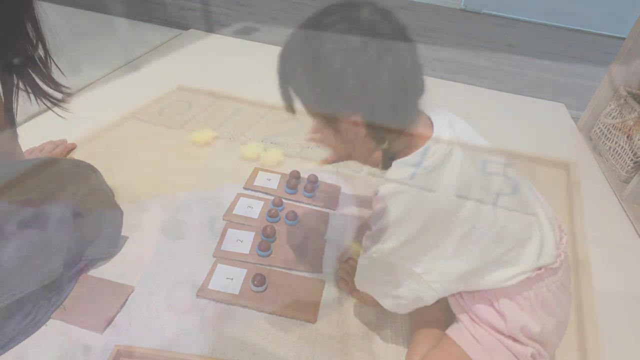 This is zero, That's right. Nothing, That's right. You can count three, One, two, three, four. One two, three, four. The next activity is cards and counters. The purpose of this material is to help children. 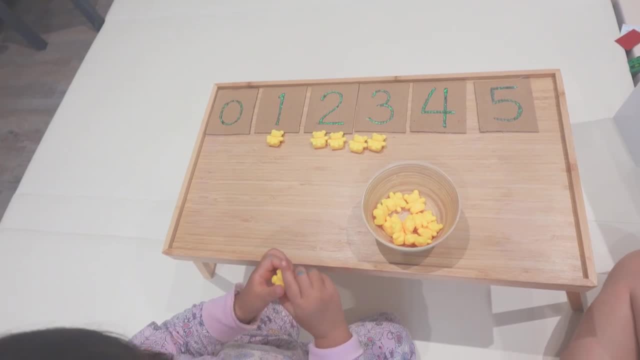 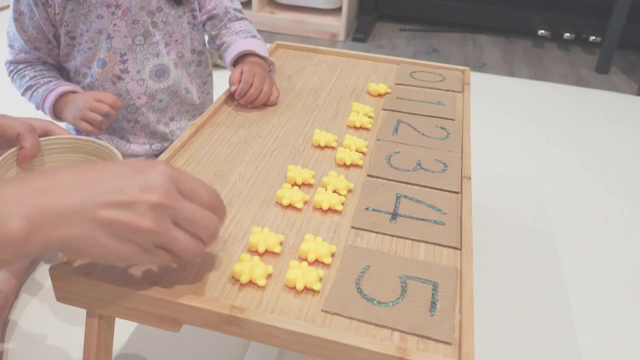 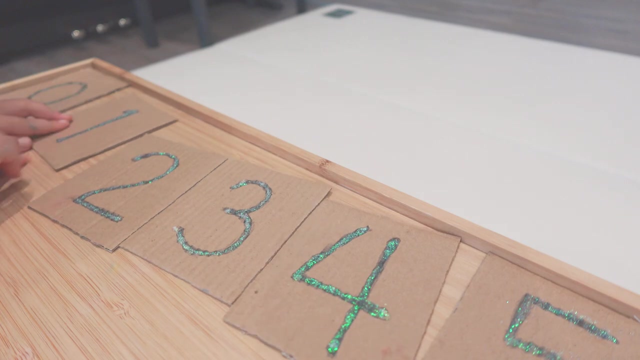 associate quantities with numbers, So your child is to place the proper quantity underneath a specific number. It's also a great way to introduce the concept of odd and even numbers. In order to DIY this material, you need your sandpaper numbers or whatever number card you have on hand, and then your counters. 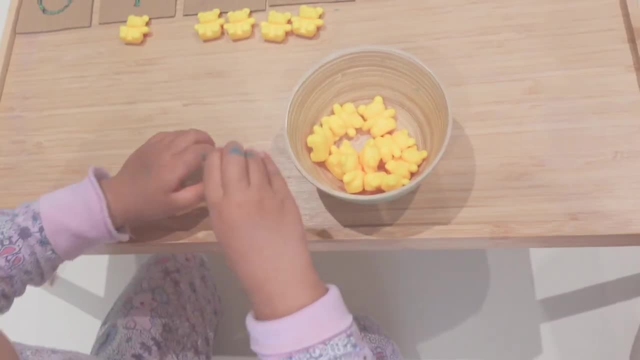 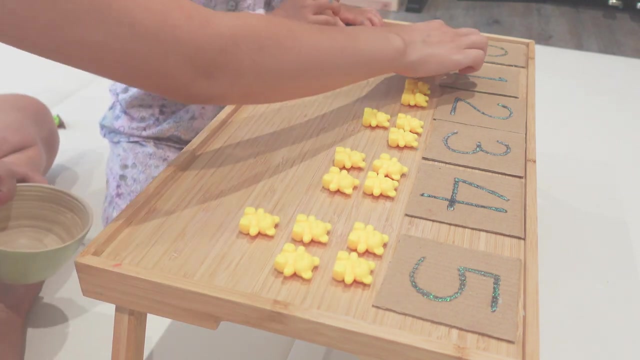 Now for your counters. make sure you have the correct number of counters to equal the exact number of cards that you have. So Alina's working one through four, Alina's working one through five, so we need 15 counters in order to be able to self-correct. 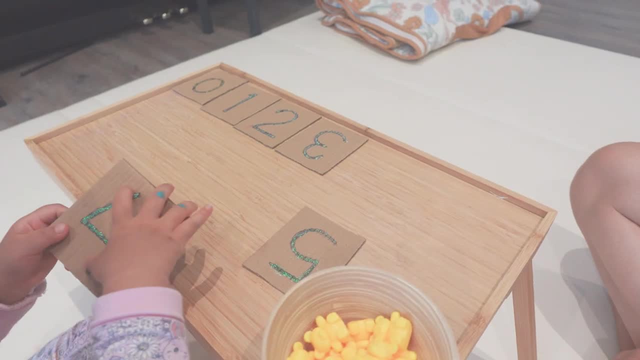 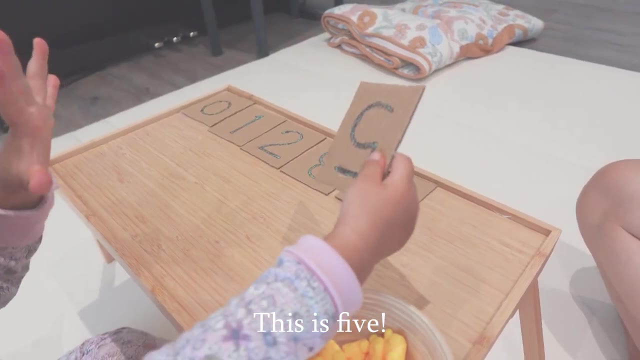 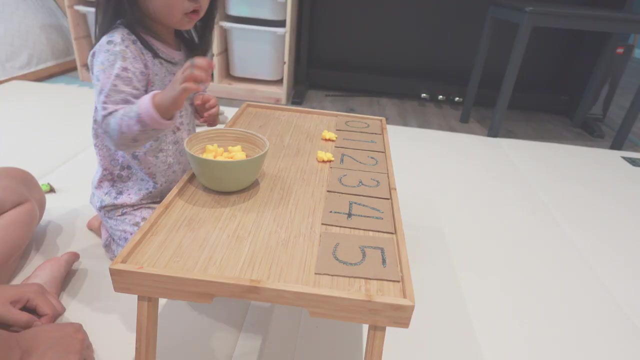 So if at the end, there are not enough, or if there are extra left over, Alina will know that there is a mistake. Now, five, Five, That's right. One, Two, Two, Mm-hmm, I think I recommend that this. 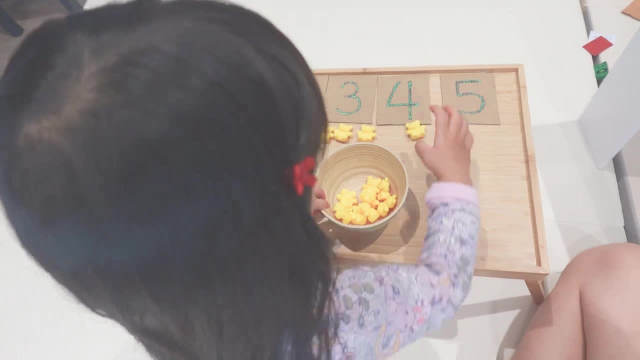 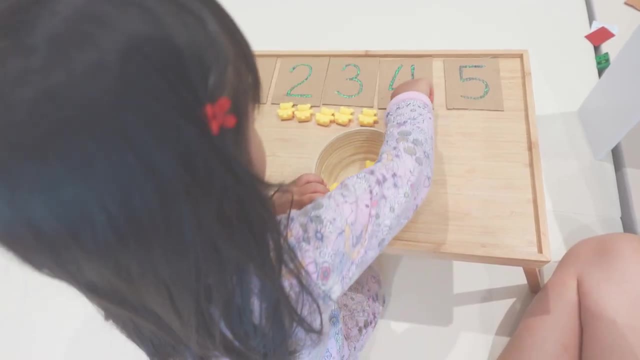 This activity be introduced a little bit later on, after your child has already had some experience with the number rods as well as the spindle boxes. I think this activity was a bit too challenging for Alina, so she kind of got distracted and then lost her interest in the middle of it and then just walked away. 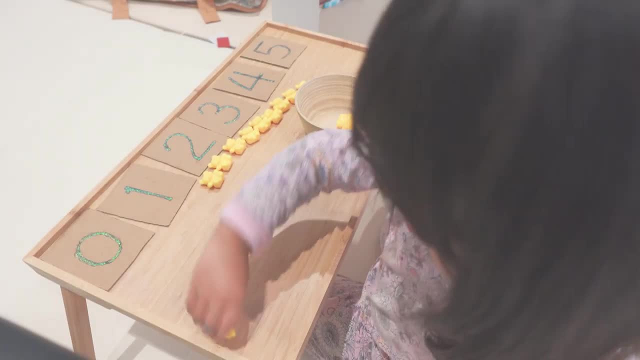 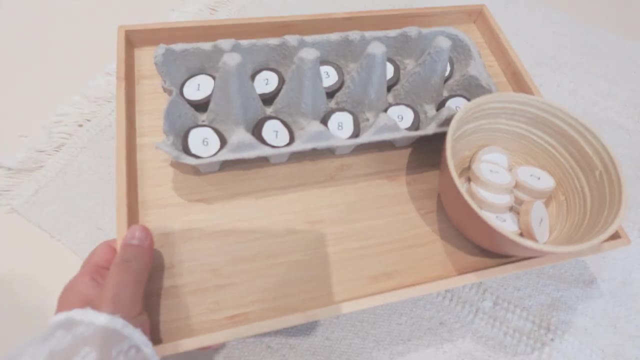 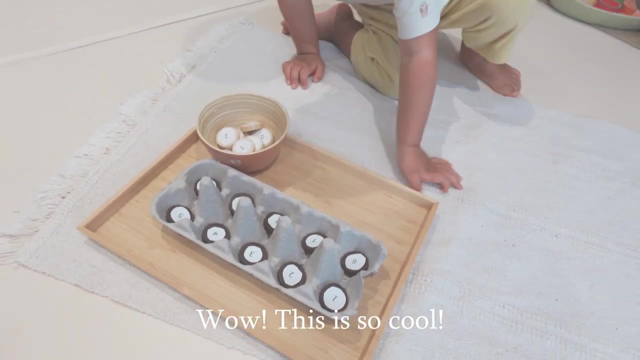 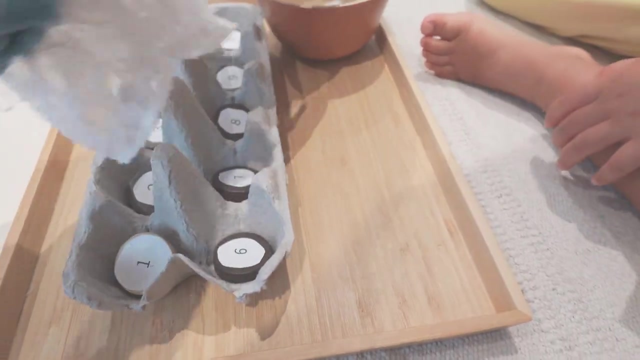 I'm holding it by myself. Is that so That one? What is that? Wow, What is this? My mom made this yesterday. Wow, It's so cool. For most children, the sensitive period for learning mathematical concepts is between the age of four and six years. 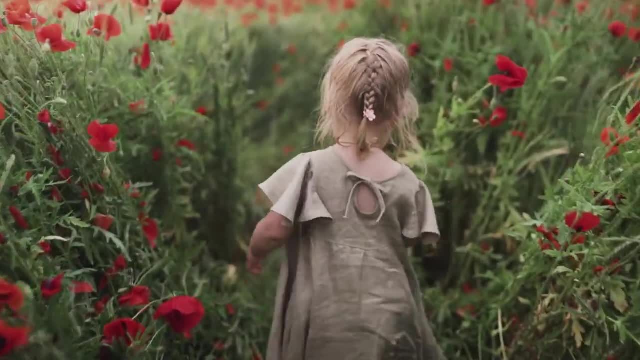 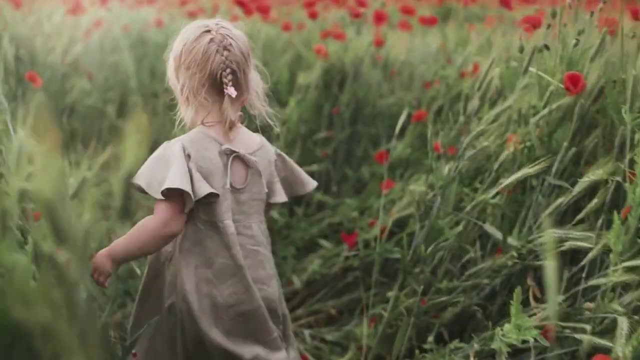 Before that, children need to develop their hands. their concentration, make sensorial impressions of the world around them. So there's no need to rush your child into learning math before they get to preschool. It's OK to just forget about it. 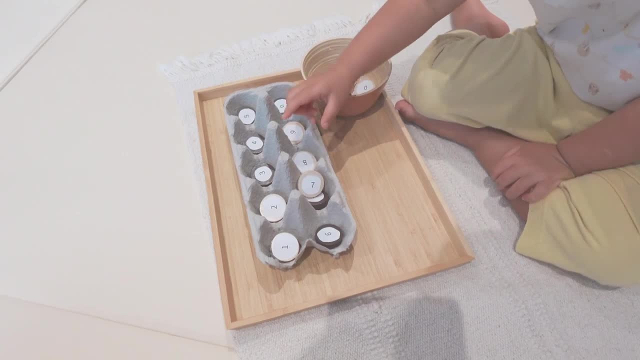 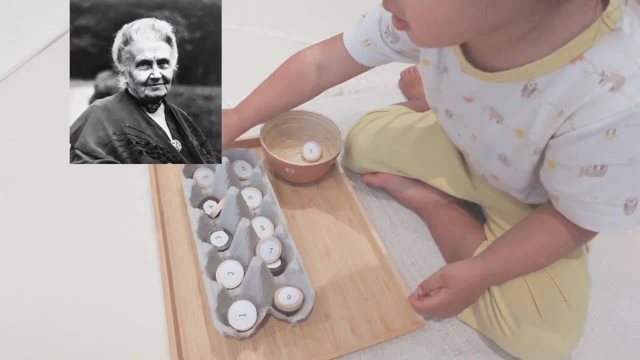 And they will learn when the time comes. But with that said, I think it's also totally fine to gently introduce some of those mathematical materials that were carefully designed by Dr Maria Montessori for the kids who are interested in numbers and counting.